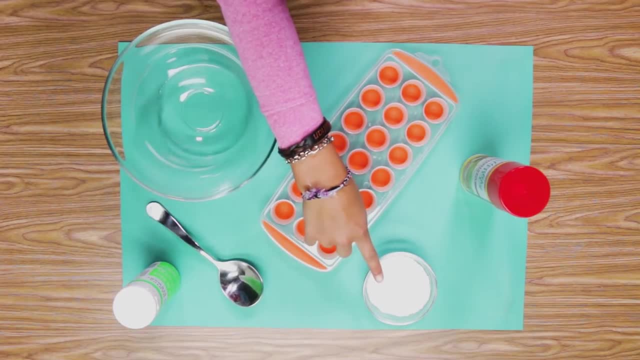 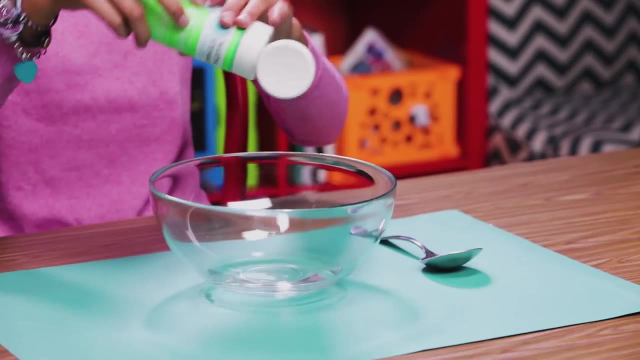 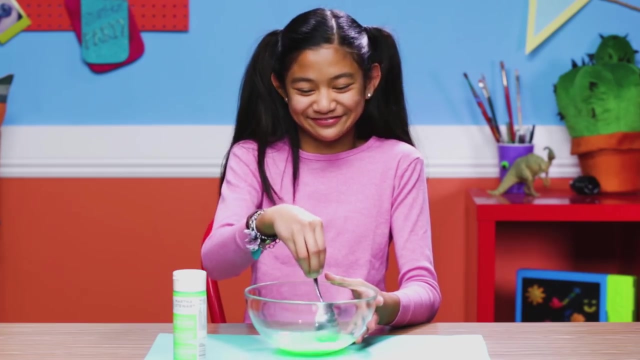 an ice tray, three tablespoons of plaster of Paris and non-stick spray. First spray your ice cube tray with cooking spray and set it aside. Add a squirt of paint to your water. Mix this together until the paint is dissolved. Add your plaster of Paris a little bit at a time. 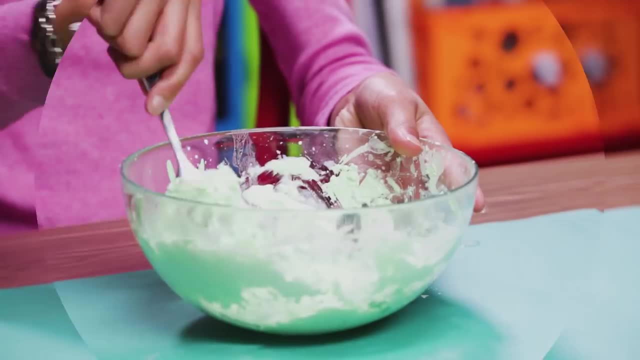 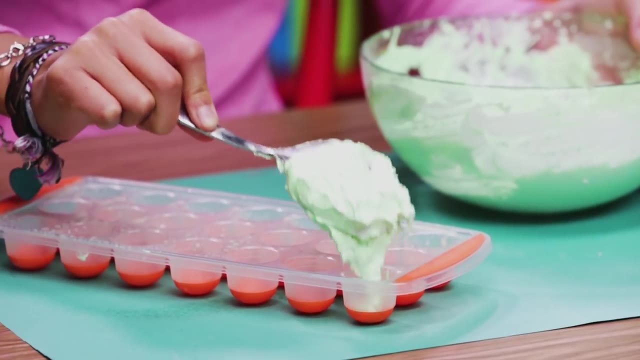 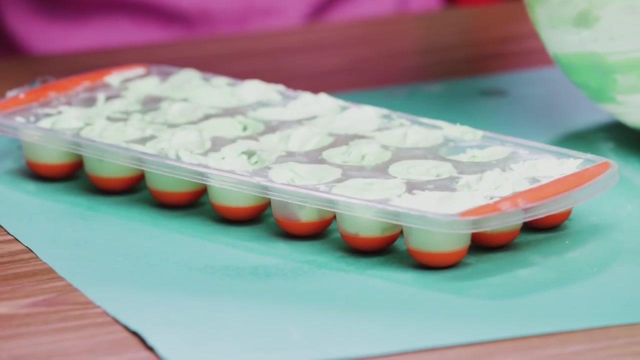 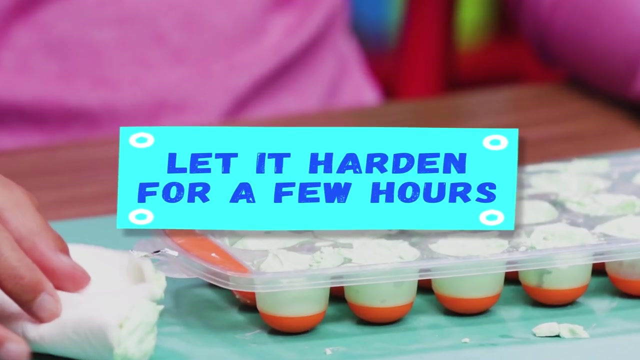 Make sure to mix while you're adding. It should be thick like this kind of like cream cheese. Once you have a thick paste, spread it into an ice cube tray. Use a paper towel to help clean up the sides. Then let this harden for a few hours. 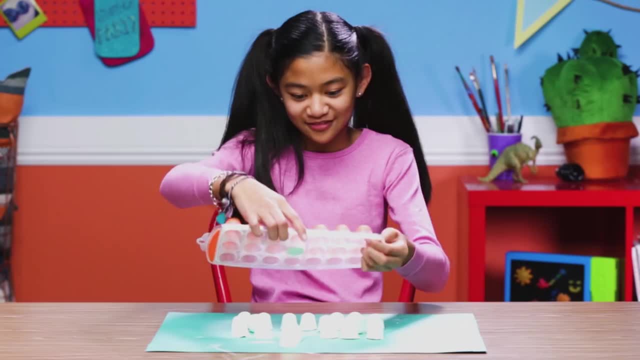 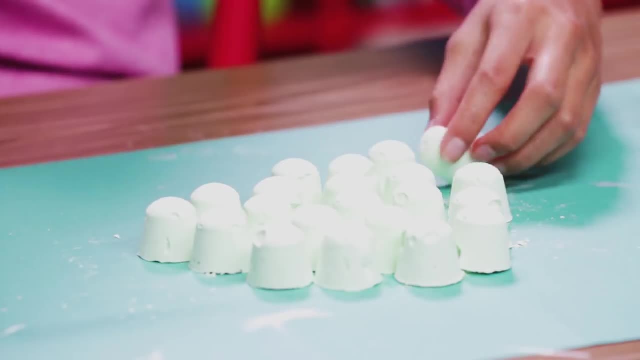 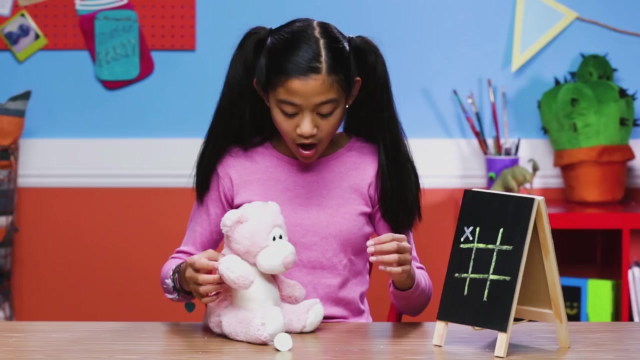 When they're hardened, pop them out. Now you're ready to write into the night. Ted, do you want to play tic-tac-toe? Here you go. Well, looks like you're good at dropping stuff, which means you'll be perfect for dropping down to the ground with my next hack. 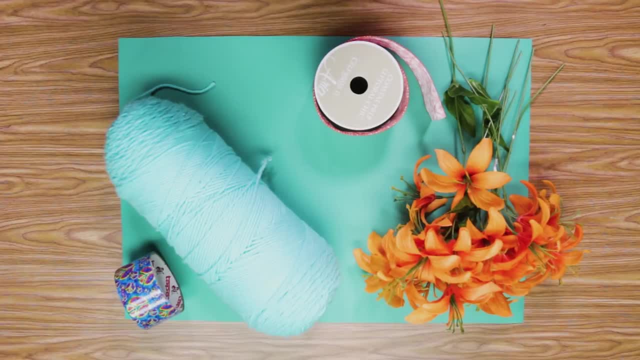 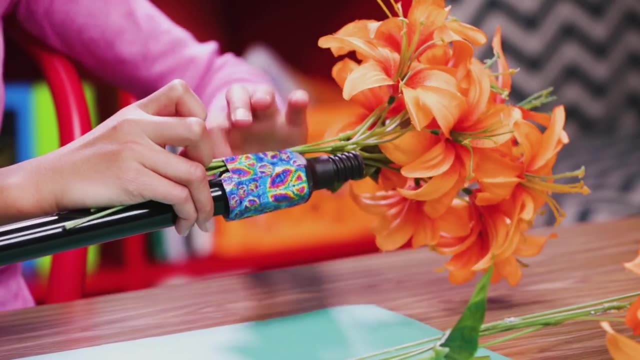 Let's make my flower power limba luau stick. For this you'll need a lot of yarn, decorative tape, flowers, ribbon and an old broom handle. First tape your flowers to the end of each side of the stick. Then tape the end of each side of the broom handle. 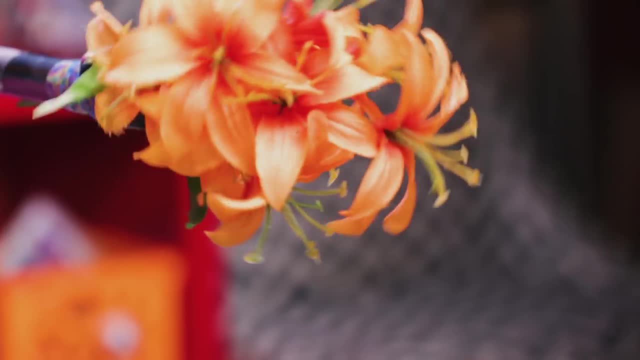 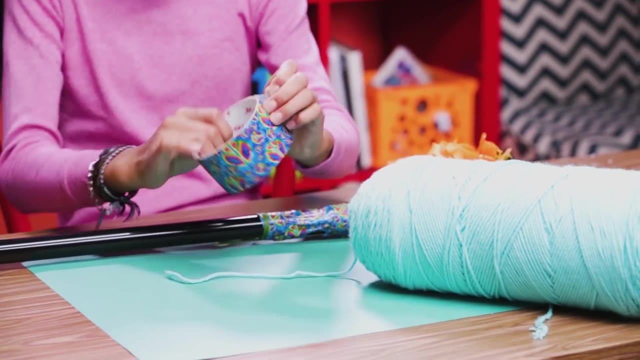 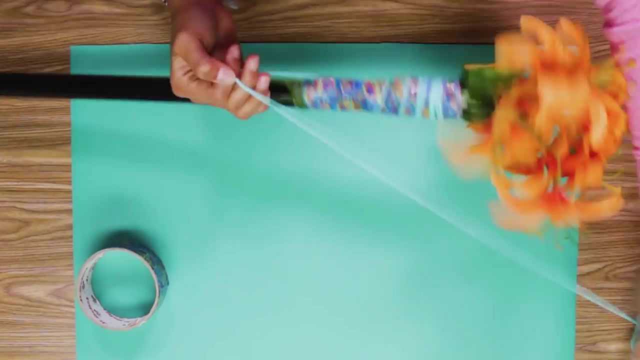 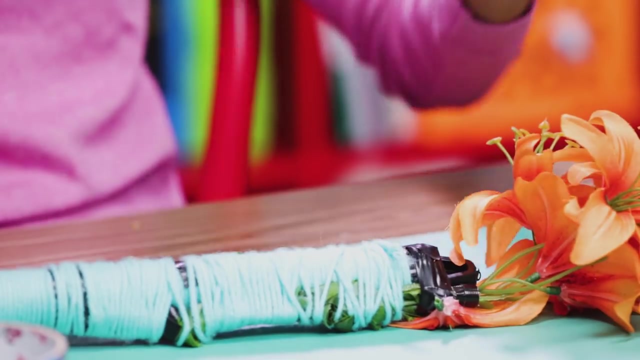 Flowers on this side and this side. Grab your yarn and tape it to one end. Start wrapping. When you get to the end, tape the yarn down. Now add some ribbon on the ends to finish it off. I'm using wire ribbon. 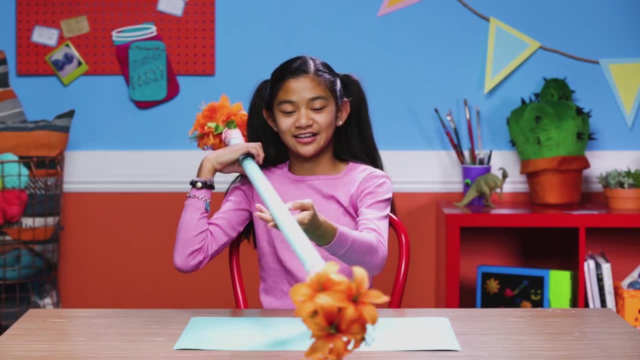 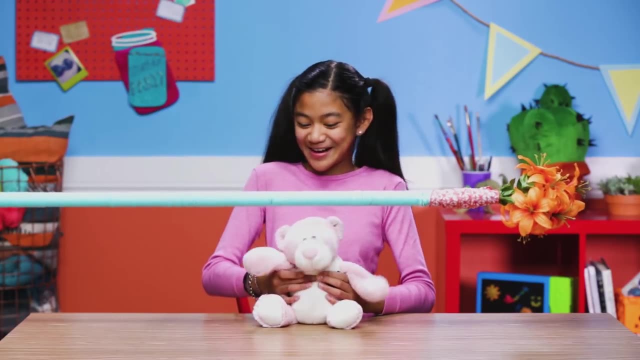 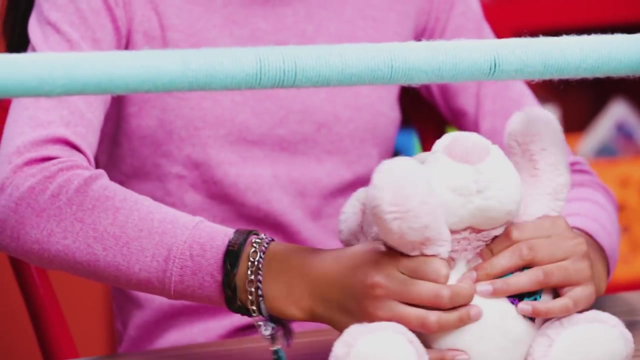 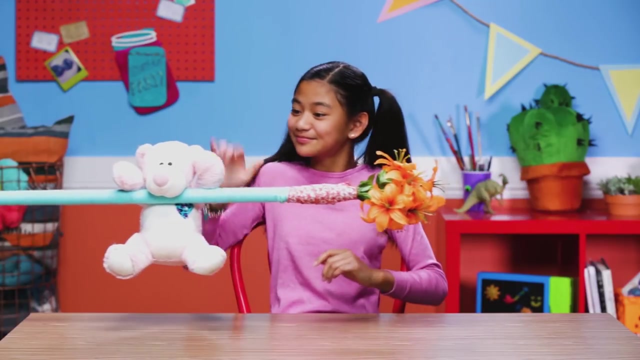 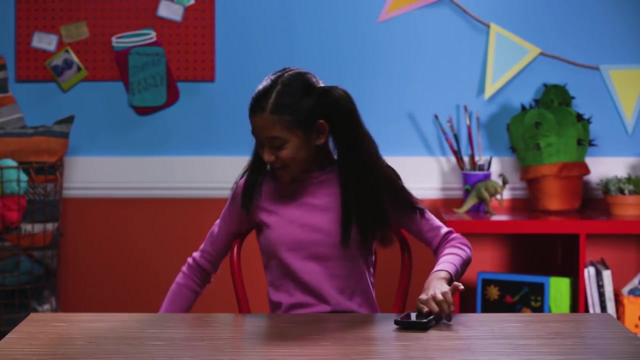 This side has a ribbon and this side. All right, Teddy, you go first. Whoa, That's the longest I've ever seen anyone limbo. But you know the best part about sleepovers: Siri lights out, Staying up all night.